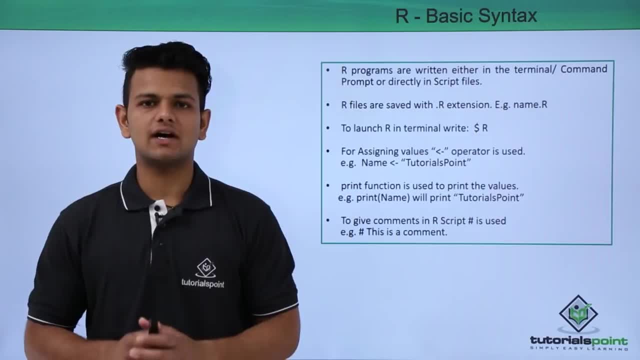 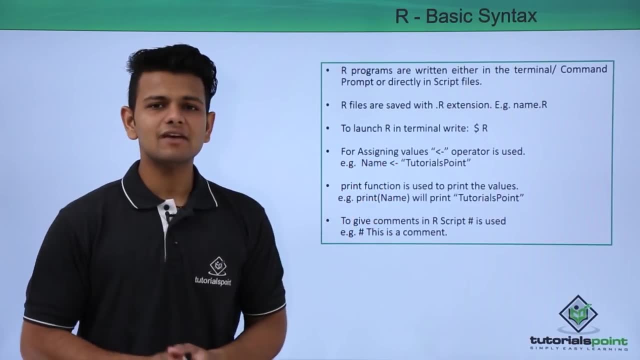 r extension. that is the file name, followed by dot r. To launch R in terminal, just write a capital R and hit enter. For assigning value: a smaller than followed by a hyphen operator is used. for example, name smaller than hyphen operator and the value that we want to assign to name. 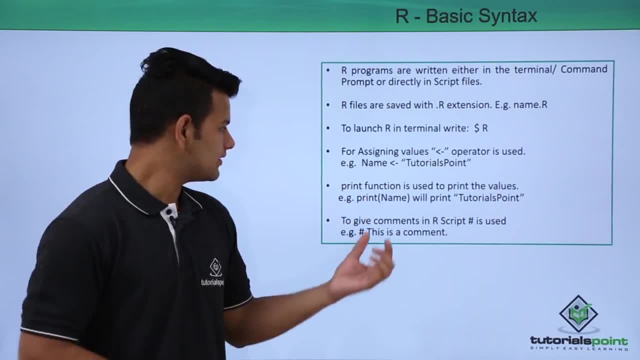 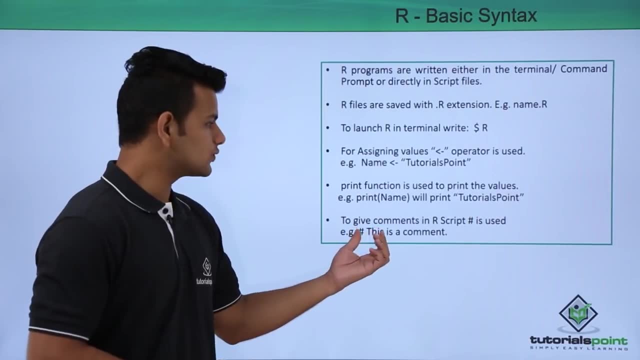 print function instead is used to print some values. for example, when we write print and name, this will print tutorials, point. that is the value stored within the name variable. To give comments in our script, hash is used, for example, hash- this is a comment- will be exactly the same as print. andly is used to print for ideas. DB teaching in R programming language. 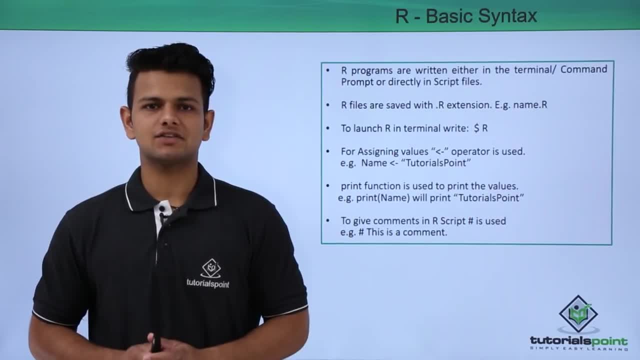 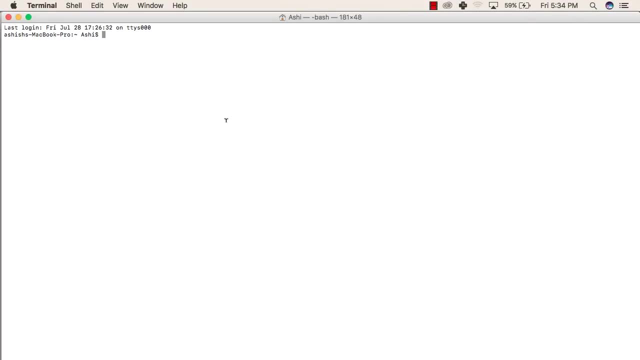 note by the compiler. now let us see a practical implementation of this basic syntax of our language. to start our compiler in your system, first go to the terminal, then press R and then press enter. this will start the our compiler. inside this you can write your our code line by line. for example in first line: 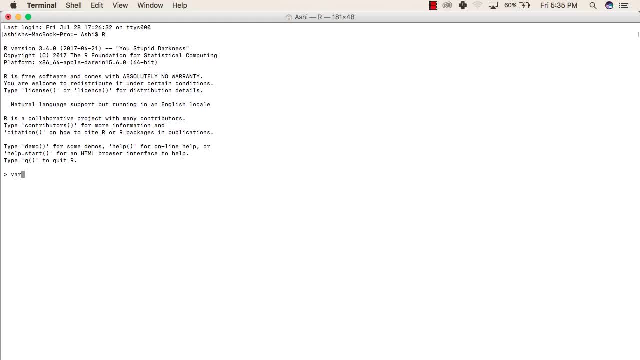 we will assign a variable, some value like where X will get some value like hello. after this, we'll print this value using the print function, so this will print hello. now we need to write a comment. this line will not print anything because the print function is written. 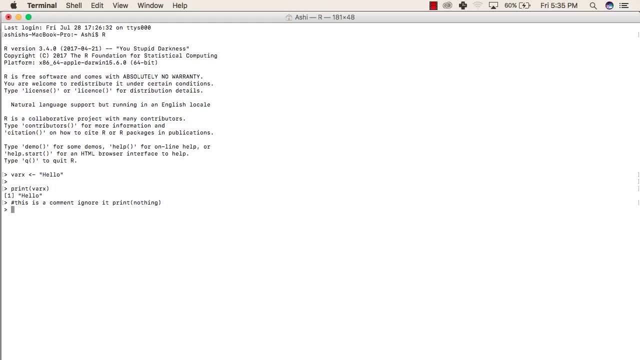 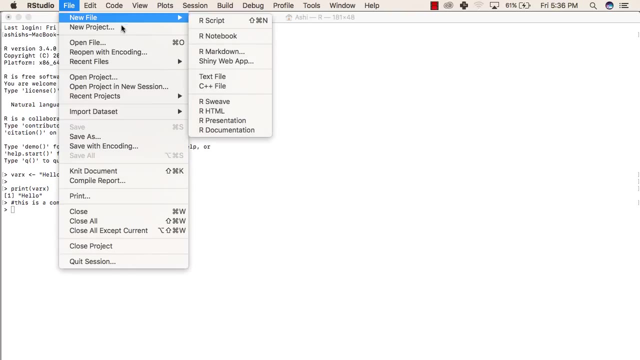 inside a comment line. as expected. this line is not printing anything. the same code can be written in our studio. for that you need to go to our studio, select file from there and new file and then select our script. now inside this file you can write the same. 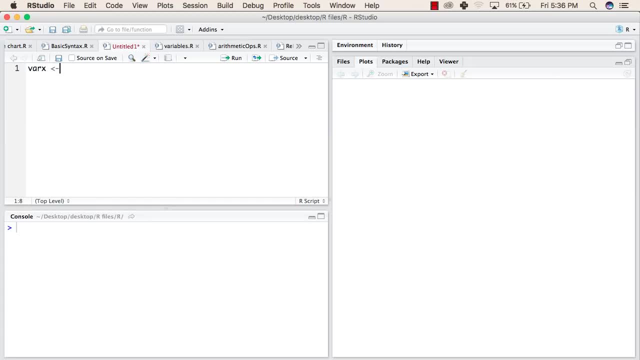 code like where X hello world. after that you will try to print this. after that you will write a comment line. now you can run this code line by line by selecting the lane and then clicking on run, or you can select the complete all the lines at one time and select run.